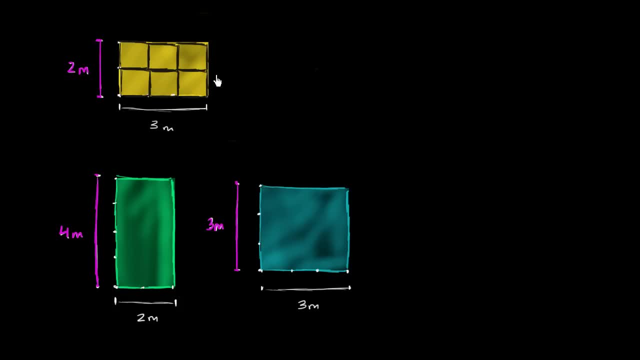 So we see here that the area is 6 square meters. Area is equal to 6 square meters, But something might be jumping out at you. Did I really have to sit and count 1,, 2,, 3,, 4, 5, 6?? 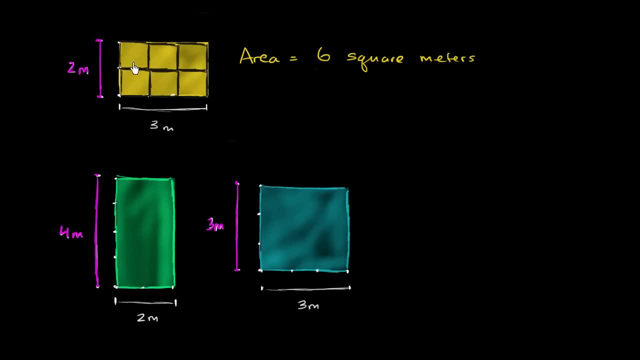 You might have recognized that I could view this as really two groups of three, And let me make that very clear. So, for example, I could view this as one group of three and then another group of three. Now, how did I get groups of three? 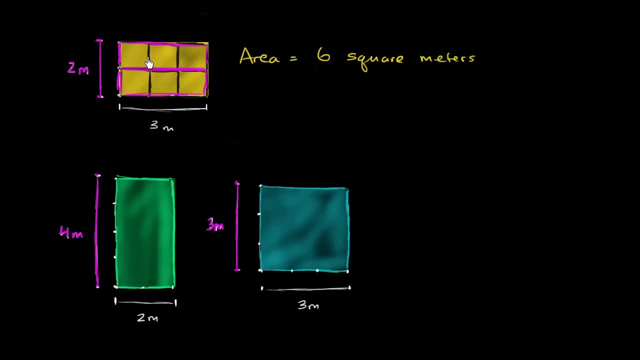 Well, that's because the width here is 3 meters, So I could put 3 square meters side by side. And how did I get the two groups? Well, it's 2 meters. This has a length of 2 meters. 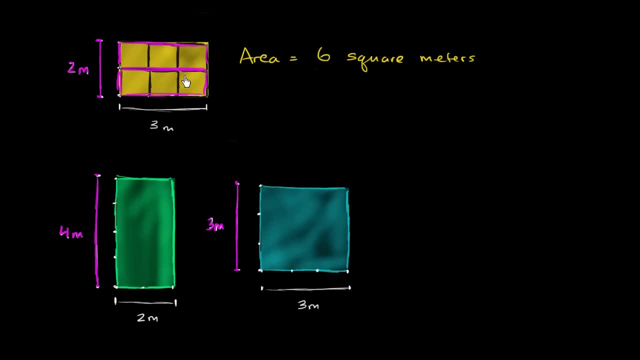 So another way that I could have essentially counted these six things is I could have said: look, I have a length of 2 meters, So I'm going to have two groups of 3.. I'm going to have 2 groups of 3.. 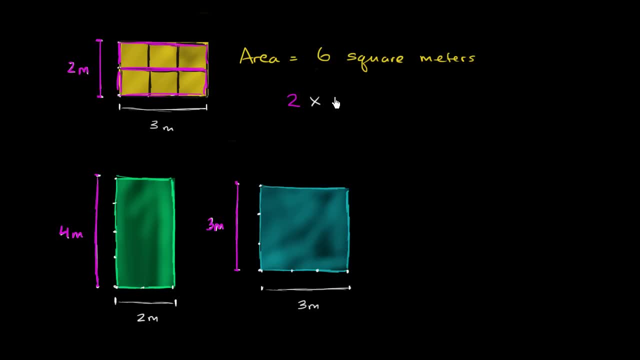 I'm going to have 2 groups of 3.. I'm going to have 2 groups of 3.. So I could multiply 2 times 3,, 2 times 3,, 2 times 2 of my groups of 3, and I would have gotten 6.. 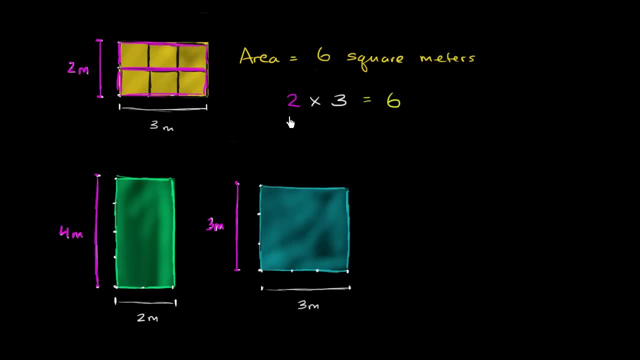 And I would have gotten 6.. And you might say, hey wait, is this just a coincidence, That if I took the height, or if I took the length and I multiplied it by the width, that I get the same thing as its area? 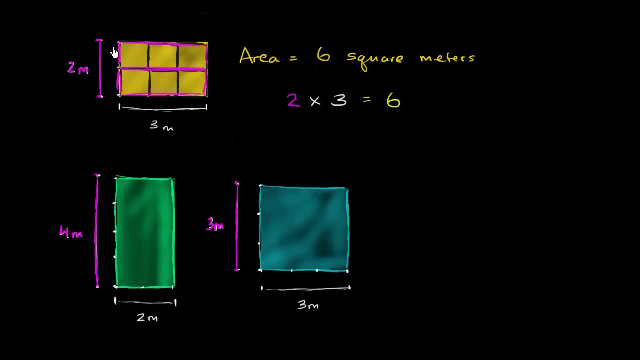 And no, it's not, Because when you took the length, you essentially said, well, how many rows do I have? And then you say, when you multiply, when you multiply it by the width, you're saying, well, how many squares do I? 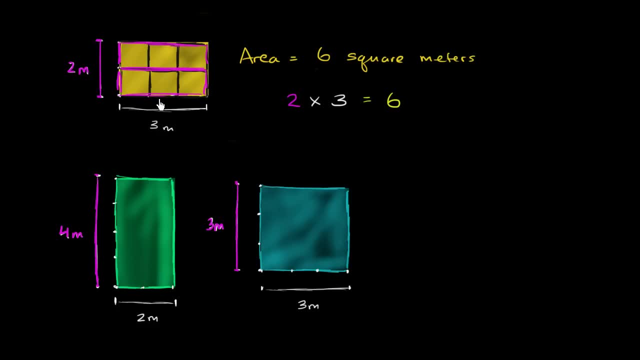 or how many of these square meters can I fit into a row? So this is really a quick way of counting how many of these square meters you have. So you could say that 2 meters multiplied by 3 meters is equal to 6 square meters. 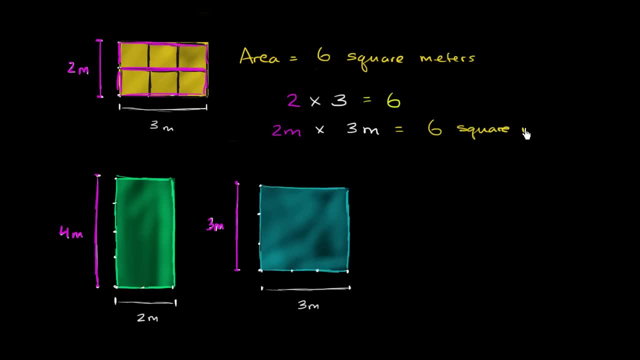 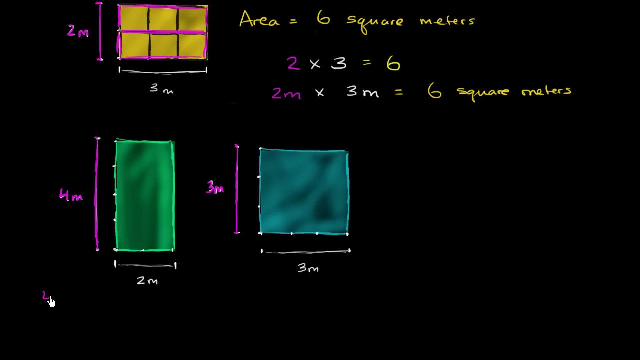 Is equal to 6 square meters. Now you might say, hey, I'm not sure if that always applies. Let's see if it applies to these other rectangles right over here. So, based on what we just saw, let's take the length: 4 meters. 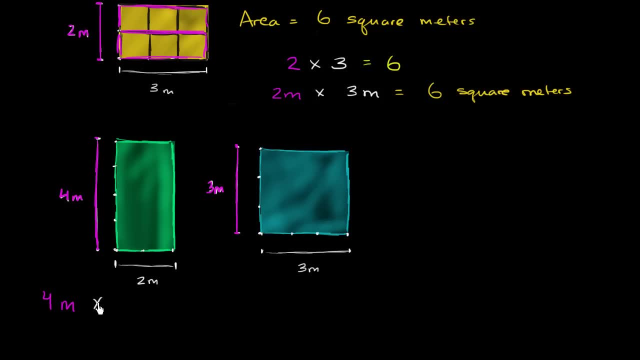 and multiply by the width and multiply by 2 meters. Now, 4 times 2 is 8.. So this should give us 8 square meters. Let's see if this is actually the case. So 1.. 1,, 2,, 3,, 4, 5.. 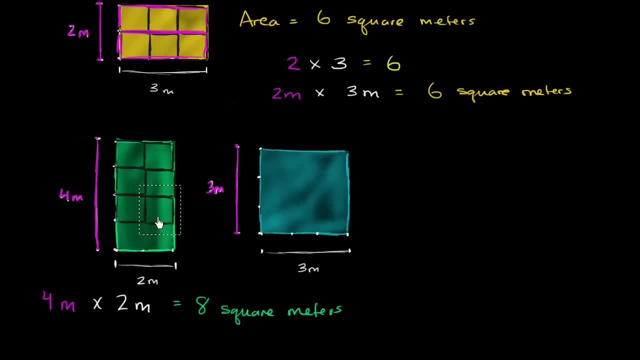 And you see it's going in the right direction. 5,, 6,, 7, and 8.. So the area of this rectangle is indeed 8 square meters And you could view this as 4 groups of 2.. So you could literally view this as 4 groups of 2.. 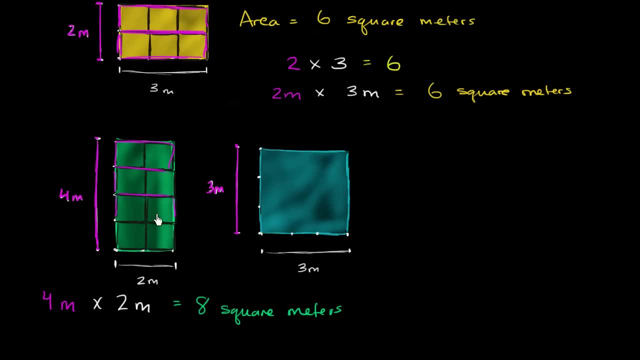 That's where the 4 times 2 comes from. So you could view it as 4 groups of 2, like this, Or you could view it as 2 groups of 4.. So 1 group of 4 right over here. 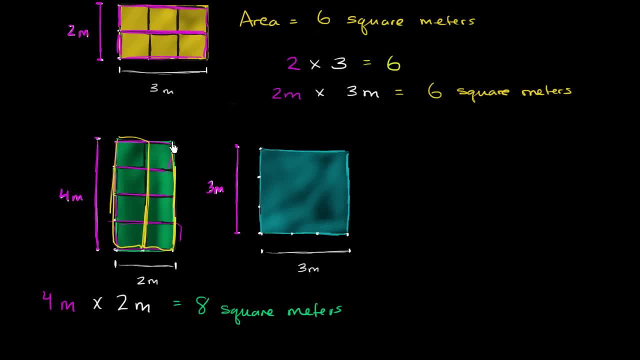 So you could view this as 2 times 4. And then 2 groups of 4.. Let me draw it a little bit cleaner Now. you could probably figure out what the area of this rectangle is. It's actually a square, because it has the same length. 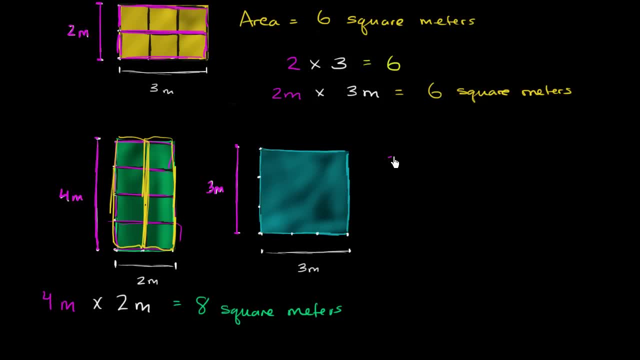 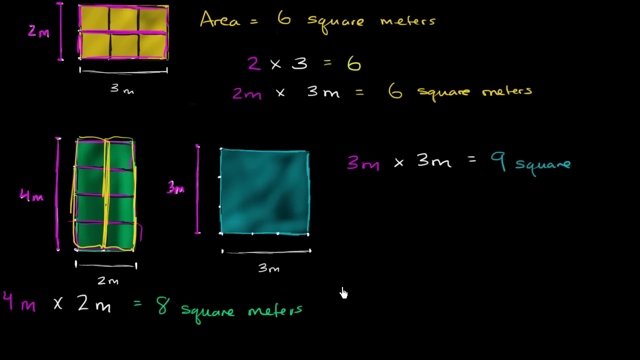 and the same width. We multiply the length, 3 meters times the width, So times 3 meters, 3 meters Meters To get 3 times 3 is 9. 9 square meters. And let's verify it again, just to feel really good. 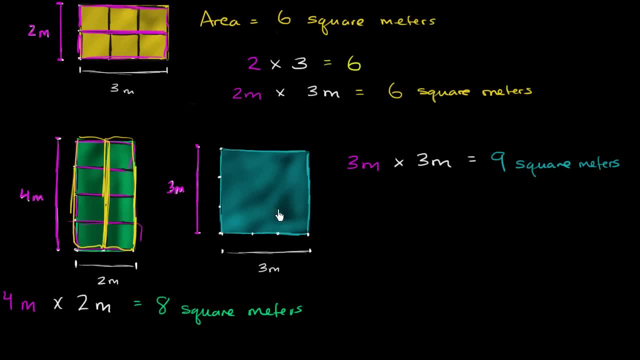 about this, multiplying the dimensions of these rectangles. So we have 1,, 2,, 3,, 4,, 5,, 6.. 7,, 8, and 9.. So it matches up. We figure out how many square meters. 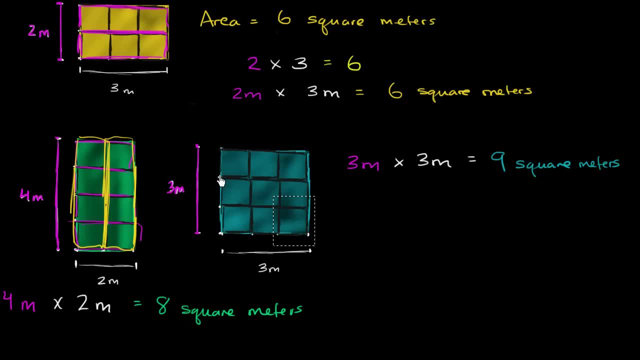 can we cover this thing with? without overlapping, without going to the boundaries? We get the exact same thing as if we multiplied 3 times 3.. If we multiplied the length times the width in meters,